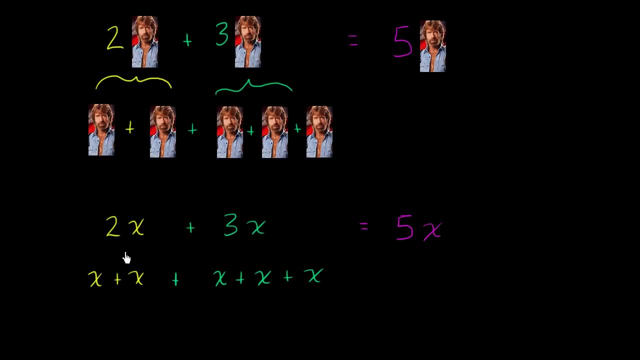 So two x plus three x is equal to five And if you think about it, all we really did- and hopefully you conceptually get it- is we just added the two numbers that were multiplying the x And these numbers, the two or the three. 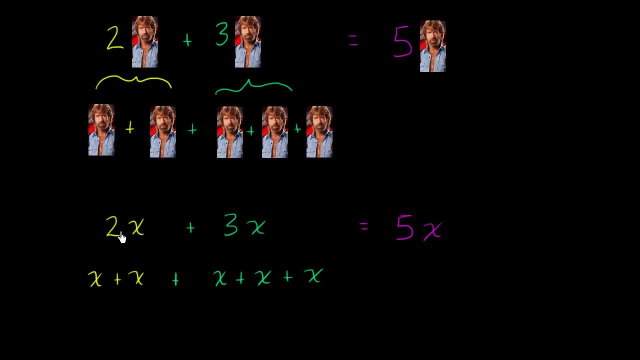 they're called coefficients- Very fancy word- but it's just this constant number, this regular number that's multiplied by the variable. You just added the two and the three to get your five x. Now let's think about this a little bit more. 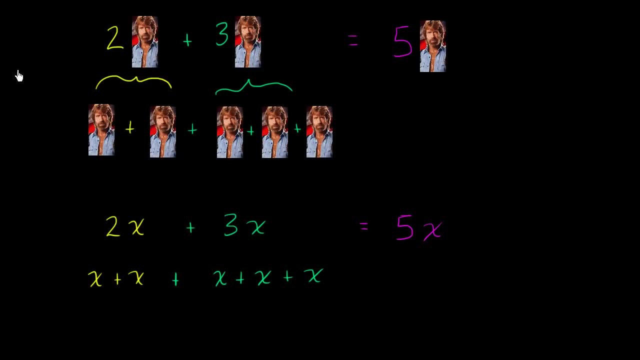 Let's go back to this original expression: the two Chuck Norrises plus three Chuck Norrises. Let's say to that we were to add. let's say we were to add some type of a. let's say we were to add seven plums over here. 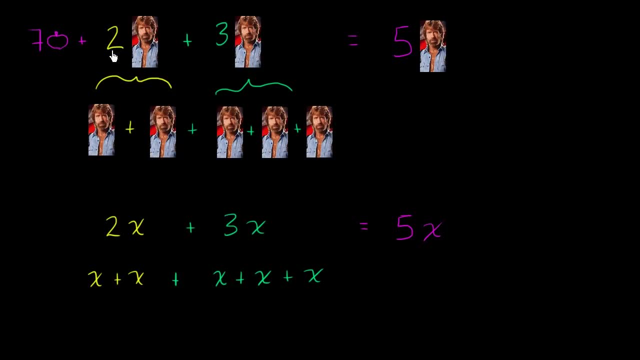 So this is my drawing of a plum. So we have seven plums plus two Chuck Norrises, plus three Chuck Norrises, And let's say that I add another two plums. I add another two plums here. So what would this whole thing be? 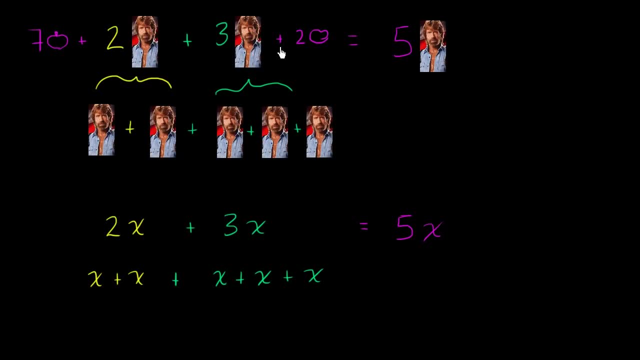 Well, I wouldn't add the seven to the two, to the three plus the two. We're adding different things here. You have two Chuck Norrises and three Chuck Norrises, so they're still going to simplify to five Chuck Norrises. 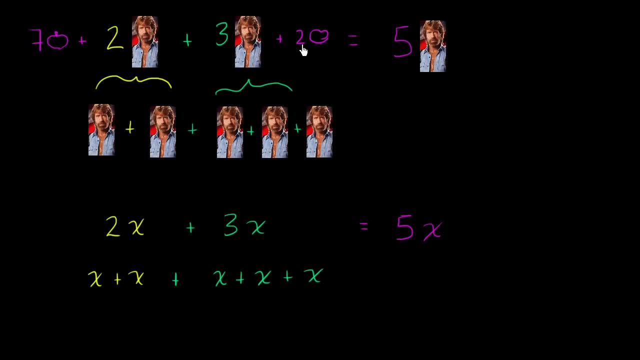 And then we would separately think about the plums. We have seven plums and we're adding another two plums. We're going to have nine plums plus nine plums. So this simplifies to five Chuck Norrises and nine plums. 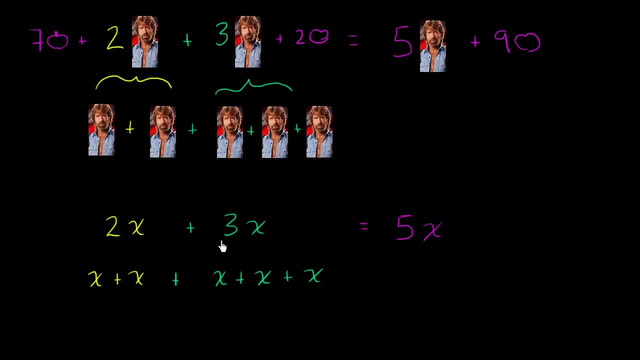 Similarly over here. if I had, instead of just 2x plus 3x, if I had, 7y plus 2x plus 3x plus 2y, what do I now have? Well, I can't add the x's and the y's. 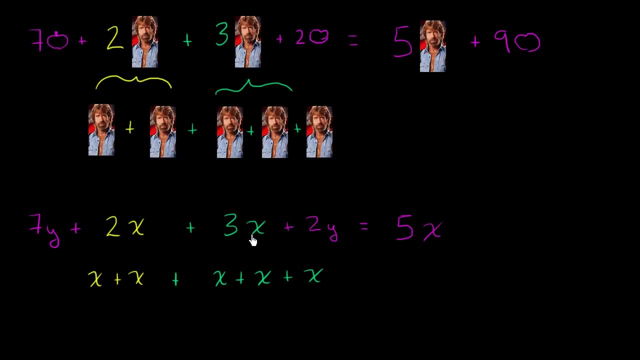 They could very well represent a different number. So all I can do is really add the x's and then I get the 5x, And then I'd separately add the y. If I have 7y's and to that I add 2y's, I'm going to have 9y's. 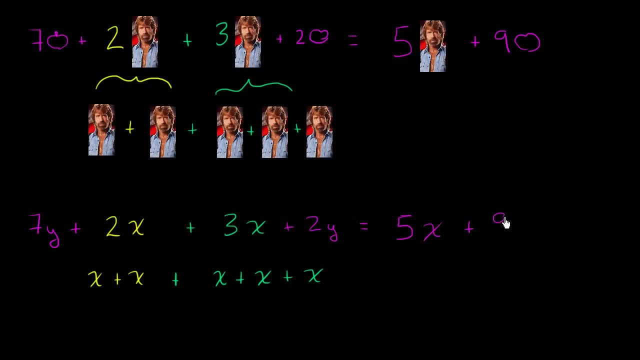 If I have 7 of something and I add 2 of something, I now have 9 of that something. So I'm going to have 9y's. So you add that and then a different color. You add this and this, you get that. 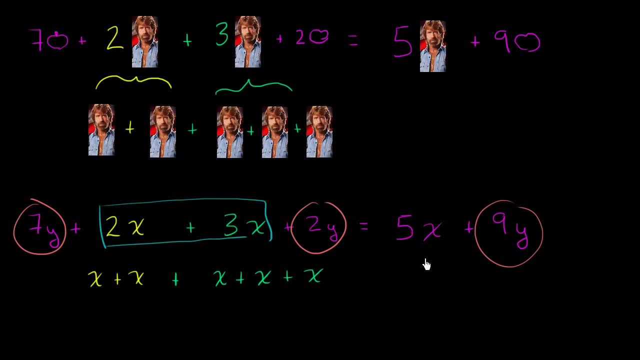 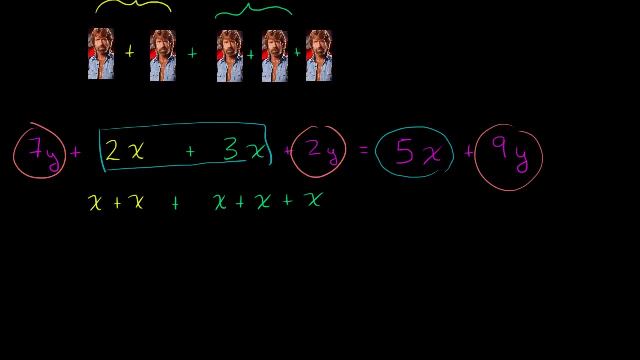 You add the x's, you get that right over there. So hopefully that makes a little sense. Actually, I'll throw out one more idea. So, given this, what would happen if I were to have 2x plus 1 plus 7x plus 5??